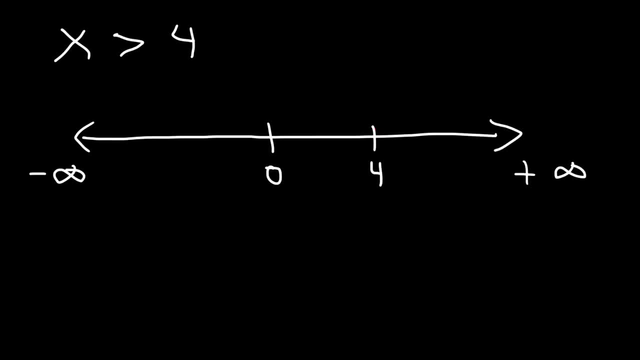 but not equal to 4, so therefore it does not include 4.. So we need to use an open circle and because it's greater than 4, we need to shade to the right Now to represent this solution, using interval notation. it's going to be 4 to infinity. 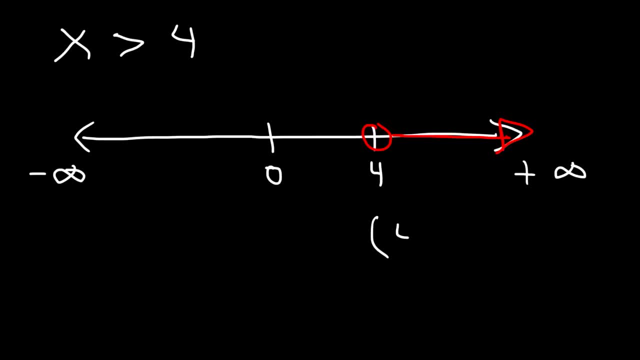 but because 4 is not included and we need to use parentheses, So 4 comma infinity. This tells us that x is greater than 4, but not equal to 4.. And so that's how you can represent this particular solution, using interval notation. Now let's try another example. Let's say: if x, 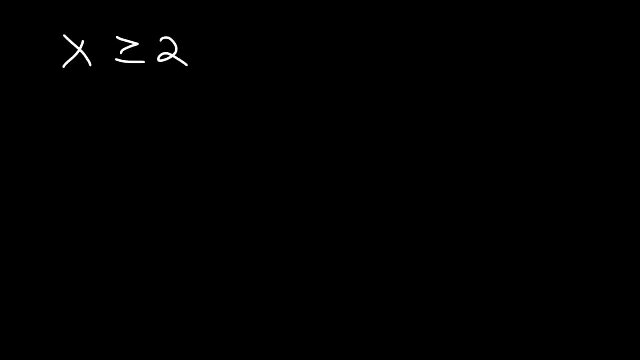 is equal to or greater than 2.. How do you think we should represent this solution using interval notation? Feel free to pause the video, Plot the solution on a number line and then write it using interval notation. So let's put 0 in the middle. 2 is to the right of 0.. On the left we're going to have negative. 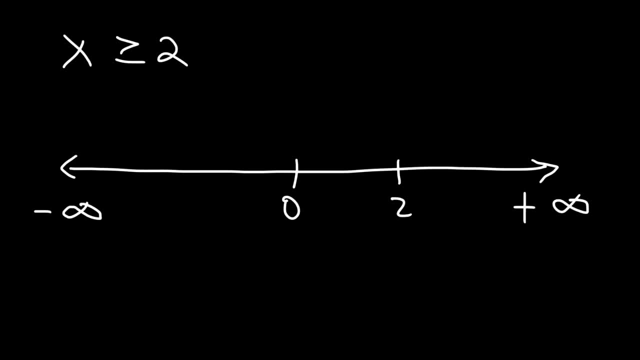 infinity as usual, and positive infinity on the right. Now, this time it's equal to or greater than 2.. So we need to use a closed circle as opposed to an open circle. but because it's still greater than 2, we're going to shade towards the right. So to 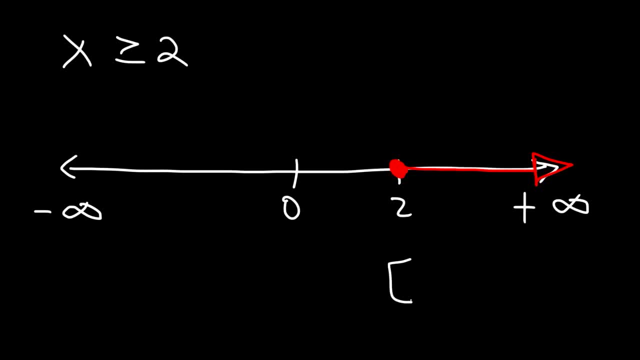 To represent this particular solution in interval notation, we're going to use brackets instead of parentheses to indicate that 2 is included. So anytime you have a closed circle, it's always going to be associated with a bracket. An open circle will always be associated with parentheses. 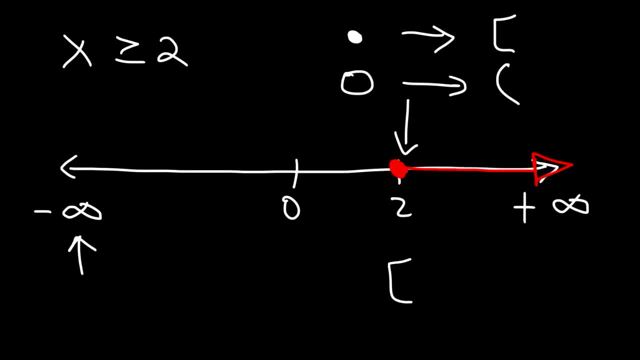 And infinity is always associated with parentheses, So it's going to be from 2 to positive infinity, And that's the answer. Now let's look at another example. Let's say that x is less than 3.. Try that one. Feel free to pause the video. 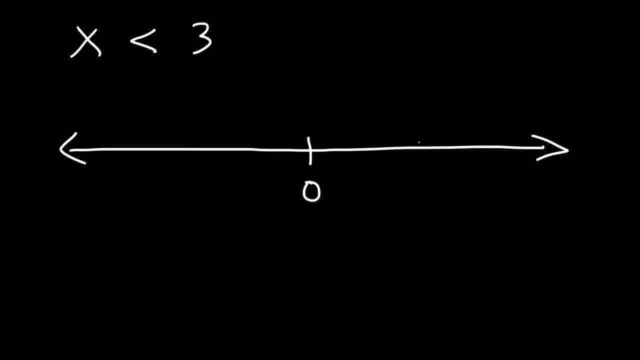 So, once again, let's start with a number line. Let's put 0 in the middle And 3 is to the right of 0. And then let's put our infinity symbols, which looks like a sideways 8.. Now x is less than 3.. 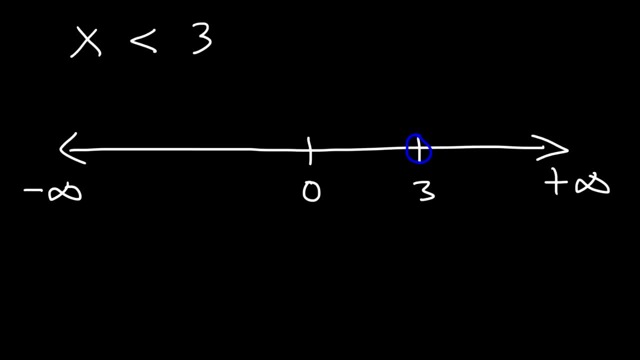 But it does not include 3.. So we're going to use an open circle at 3. But because it's less than, we're going to shade this time to the left as opposed to the right. Now, when you need to write the answer in interval notation, you should write it from left to. 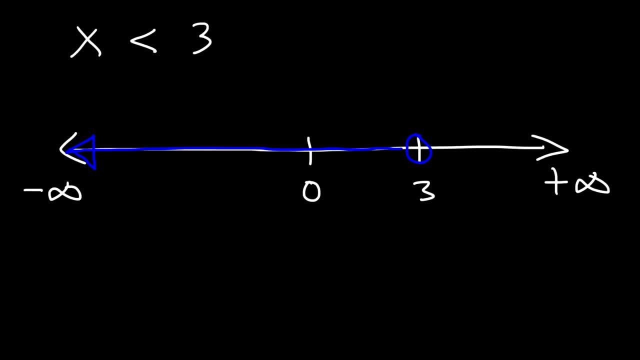 right. Basically, just write the way you see it. So the first number is negative infinity. That's the number on the left. The number on the right where the blue line ends is negative infinity. The number on the right where the blue line ends is negative infinity. 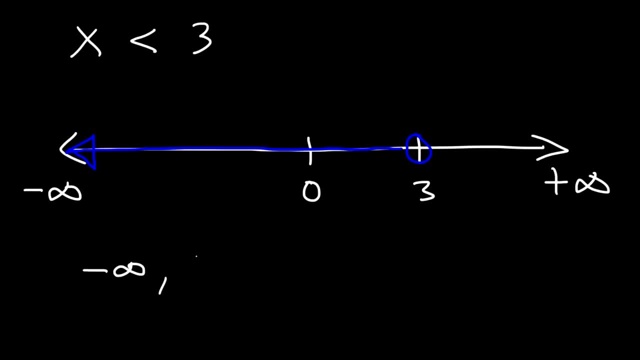 The number on the right where the blue line ends is 3.. So it's from negative infinity to 3.. Now, as we said before, you should always use a parenthesis symbol next to an infinity symbol, And we have an open circle, so that's going to be associated with a parenthesis. 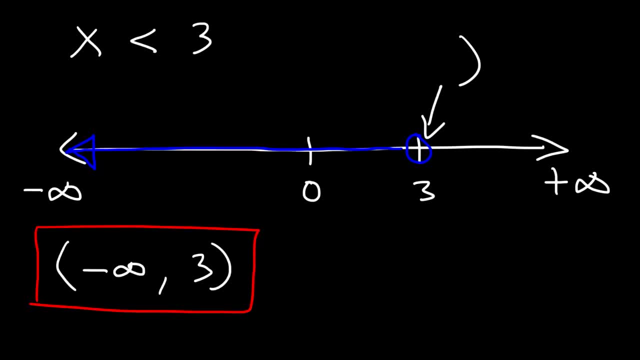 So this is the answer. It's negative infinity to positive 3.. Try this one. Let's say that x is less than or equal to negative 1.. Let's say that x is less than or equal to negative 1. Let's say that x is less than or equal to negative 1.. 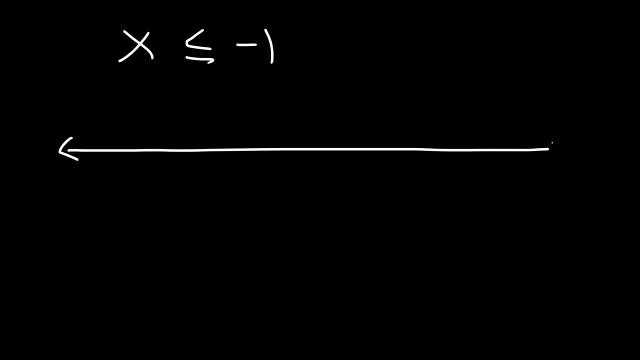 We can do this in just a minute and work on that. So let's start with a number line. So here's 0. Negative 1 is to the left of 0. Let's put the infinity symbols, so this time it includes negative 1, so we're going to. 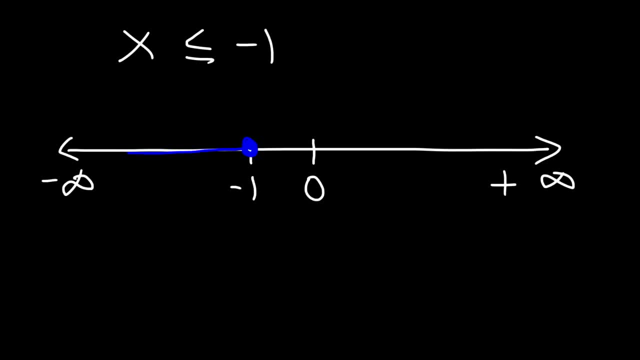 use a closed circle And because it's less than negative 1, let's shade to the left. So the left side has negative infinity and the right side has negative 1.. So we're just going to rewrite that here: Negative infinity to negative 1.. 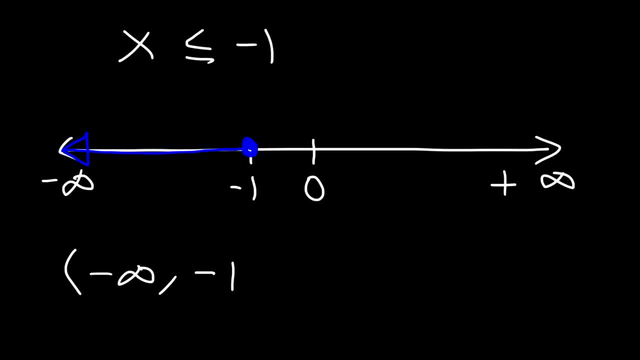 Now use parentheses always for an infinity symbol and because we have a closed circle, this is going to contain a bracket. So it's from negative infinity to negative 1, including negative 1.. Now let's work on a different type of example. 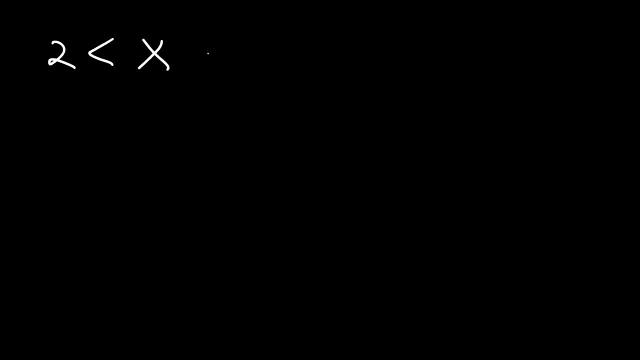 Let's go over compound inequalities. So let's say X is greater than 2, but less than or equal to 6.. Write the solution on a number line and describe it using interval notation. So let's start with 0.. 2 is to the right of 0, and 6 is to the right of 2.. 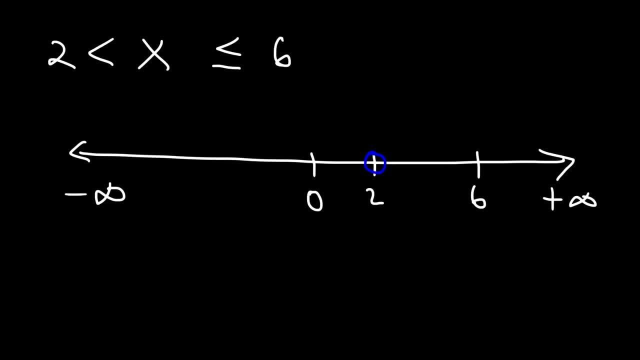 So X is greater than 2, but not equal to it. so we need to use an open circle, And 2 is to the left of 2, and 6 is to the right of 2.. So X is greater than 2, but not equal to it, so we need to use an open circle. 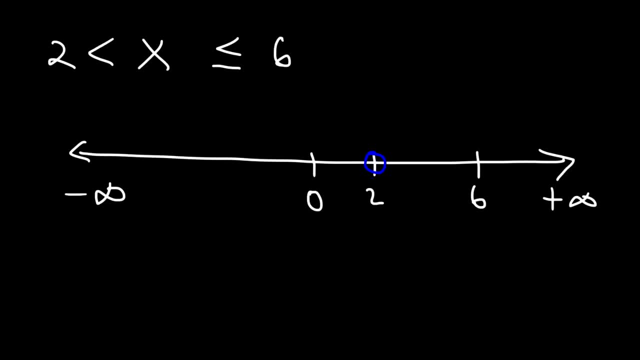 And should we use an open circle on 6, or a closed circle? What would you say? It's less than or equal to 6,, so we're going to use a closed circle at 6.. Because it's less than 6,, we need to shade to the left. 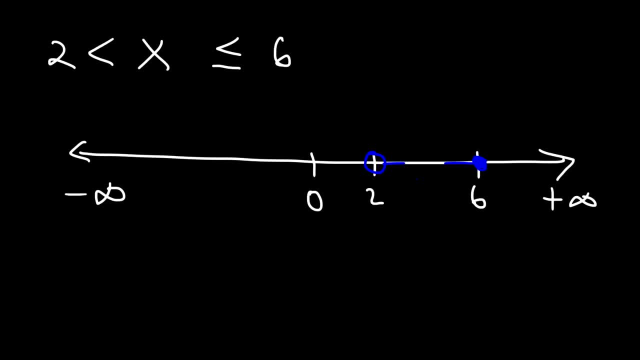 But because it's greater than 2, we need to shade to the right. Therefore, we have to shade between 2 and 6.. Now how can we represent the solution in interval notation? So the left side has a 2,, the right side has a 6.. 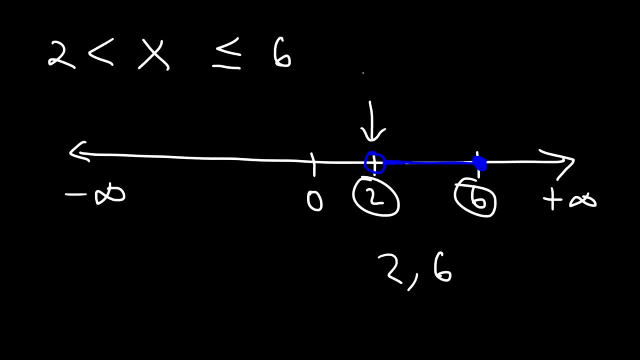 So it's going to be 2, 6.. But we have an open circle here and we have a closed circle on the right side. So for an open circle, use parentheses. For a closed circle, use a bracket. So this is the answer: 2 to 6.. 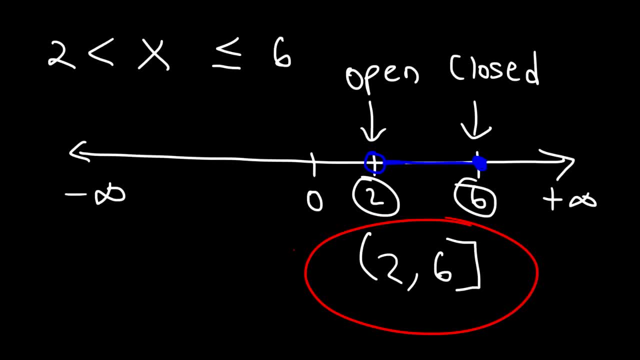 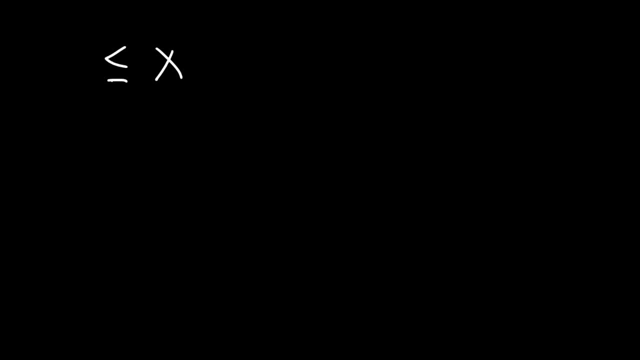 That's how you can represent it using interval notation. Now let's try another example. Let's say that X is greater than or equal to negative 3,, but it's less than 4.. Feel free to pause the video. Try that problem. 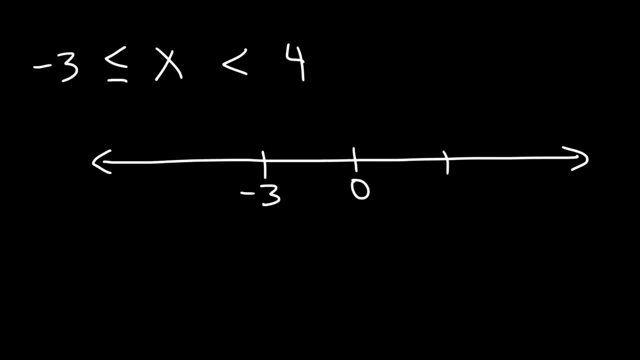 So negative 3 is to the left of 0, and 4 is to the right of it. So we're going to have a closed circle at negative 3, but an open circle at 4.. So it's greater than negative 3, but less than 4.. 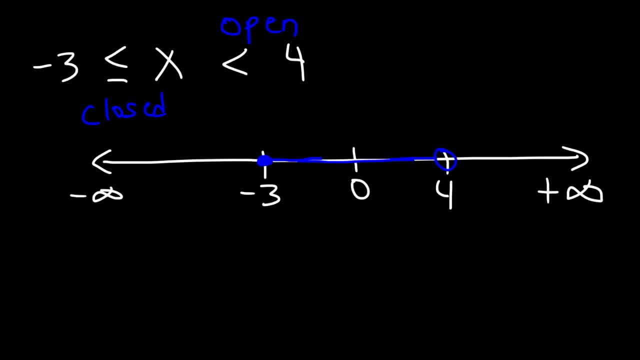 So we're going to shade to the right of negative 3, but to the left of 4.. So it's between these two. In interval notation the answer is going to be negative 3, 4.. We're going to start from the left and end on the right. 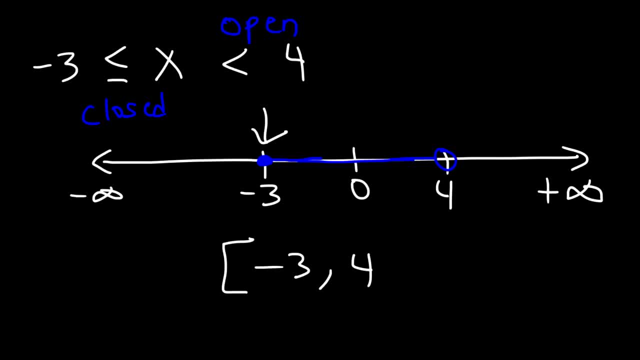 Now we have a closed circle here, so this is going to be a bracket and this is an open circle, so we need parentheses. So that's the answer: negative 3 to 4.. Now here's another example for you. 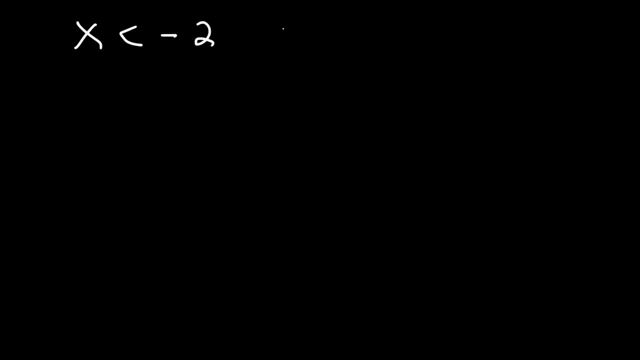 Let's say that X is less than negative 4.. Let's say that X is less than negative 2, or X is greater than or equal to 5.. Try that one. So let's start with a number line. So let's put 0, negative 2 is on the left, 5 is on the right. and then let's put our. 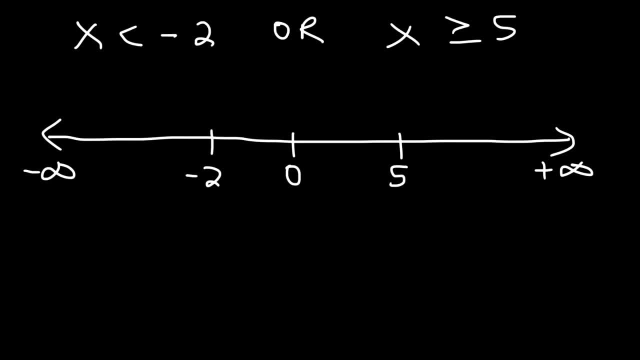 infinity symbols. Now, X is less than negative 2. So we're going to have an open circle, but because it's less than we're going to shade to the left, Or X can be equal to or greater than 5, so therefore we have a closed circle. but 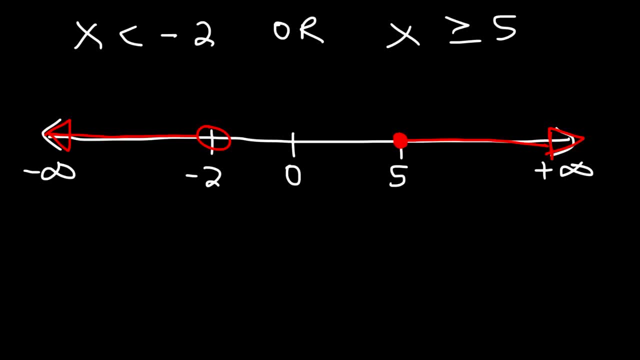 because it's greater than we're going to shade to the right. Now, how can we represent this particular solution using interval notation? So let's start from left to right. So let's focus on the left side. On the left of that portion, we have negative infinity, and then we have negative 2.. 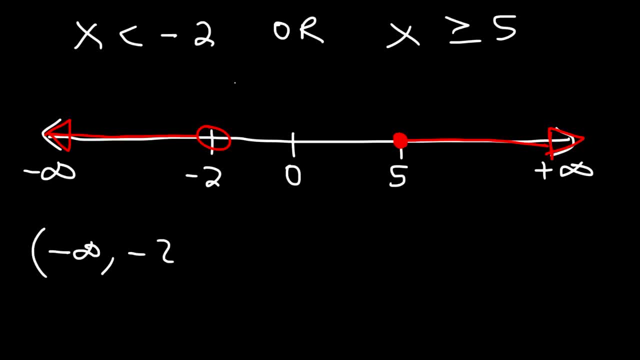 Now, with infinity, you should always use a parenthesis symbol And because we have an open circle, there's going to be a parenthesis associated with negative 2. Now to jump from this section all the way to that section and to skip everything in. 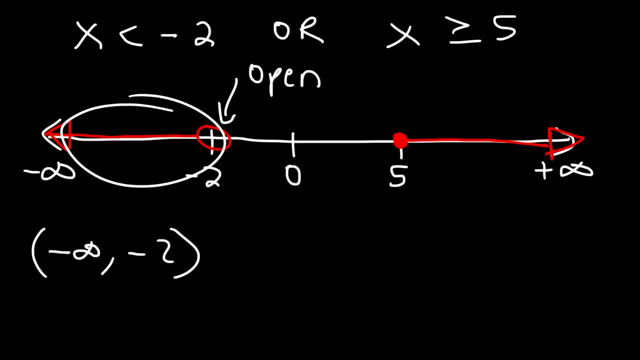 the middle. we need to use a union symbol to connect these two together. Now it includes 5, we have a closed circle at 5, so therefore we need to use brackets for 5. And then for infinity, we're going to use an open circle. 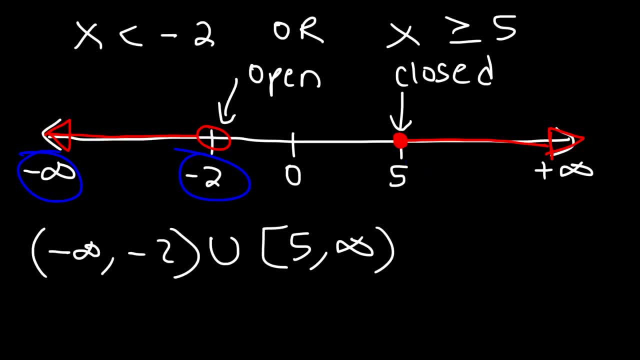 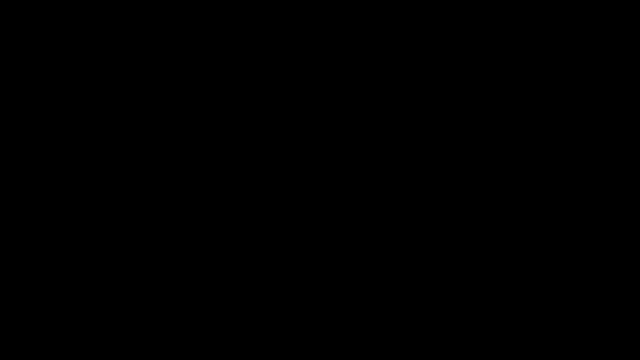 So you can literally see the numbers that you need to use in interval notation, But if you have two separated parts, connect them with a union symbol, And so this is the answer: It's negative infinity to negative 2, union 5 to infinity.